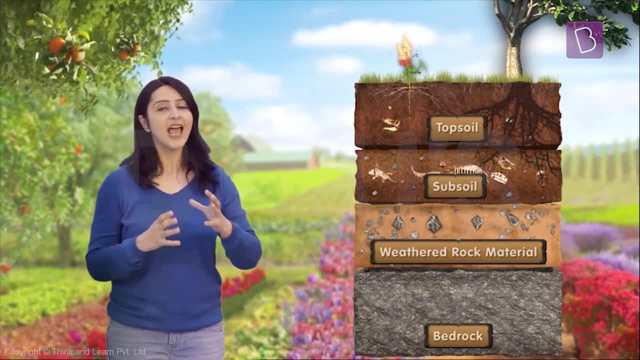 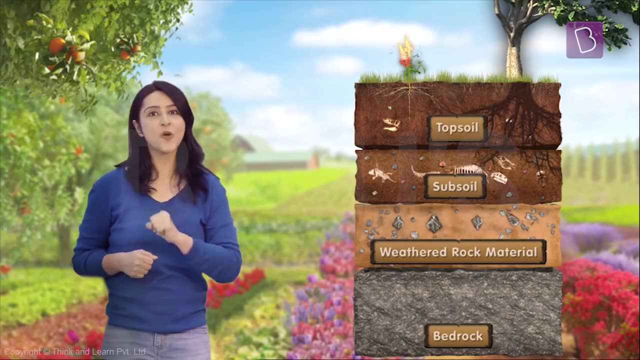 of minerals, water, humus and rock particles. But how did such diverse components come together to form soil? Soil formation starts with the weathering of rocks. Rocks are exposed to water through tidings and by the then saddledge. There are Lunch Нä ε super surface earth space 녹я 곯. 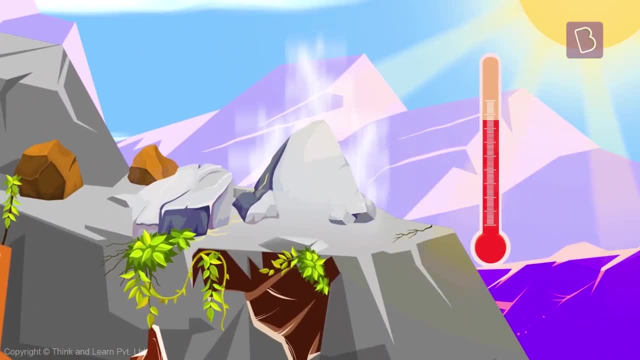 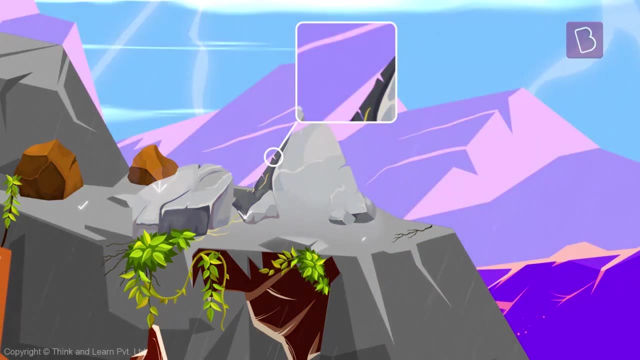 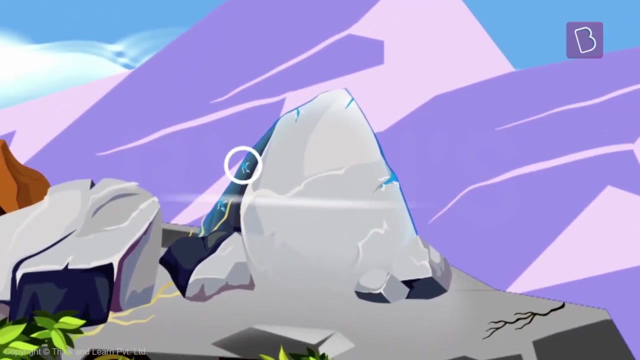 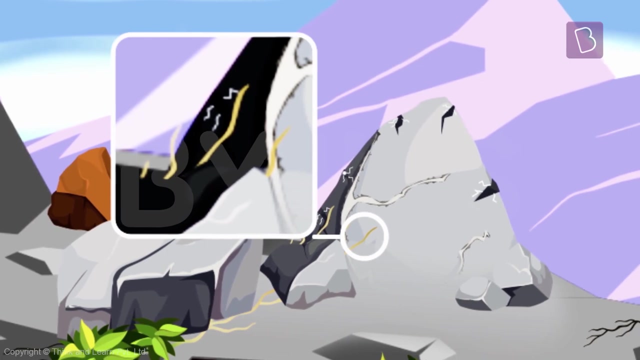 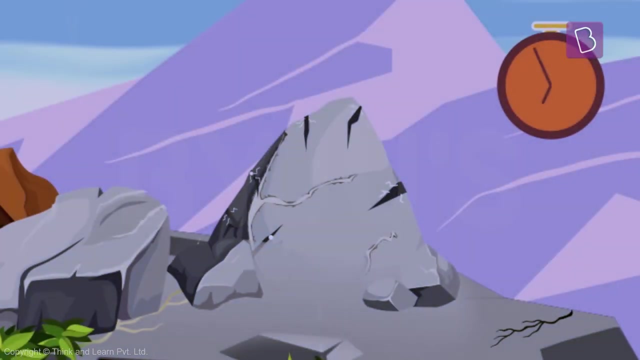 pping nä. to temperature changes, undergo expansion and contraction and start cracking. over time, Rainwater enters these cracks and becomes ice. when the temperature drops, The ice widens the cracks further. Sometimes the roots of plants also cause cracks in the rocks. Slowly over a period of time, the rocks break and 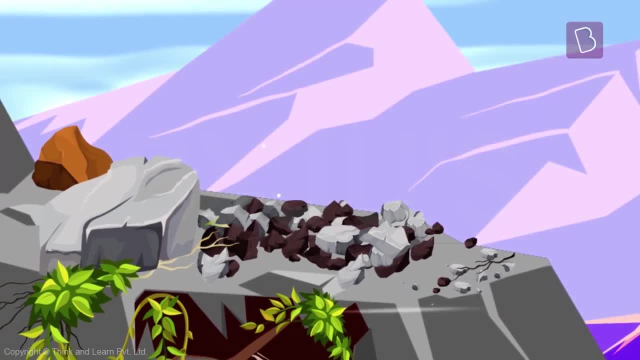 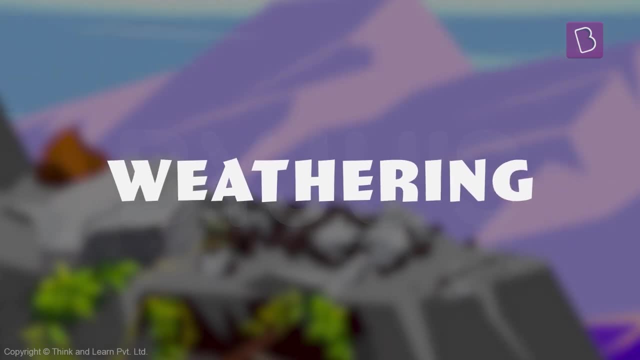 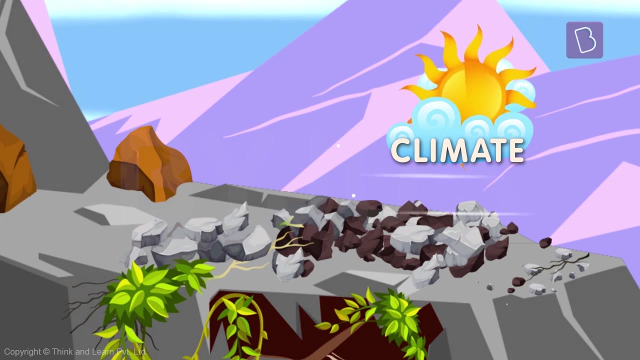 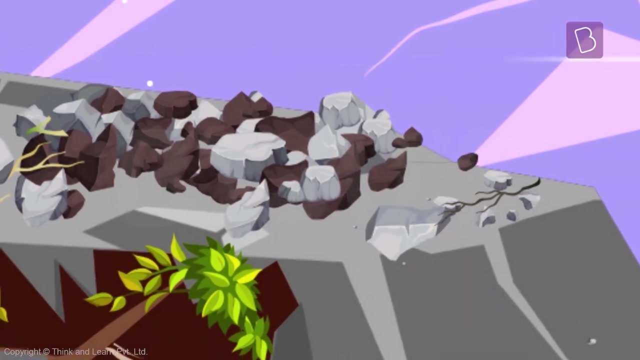 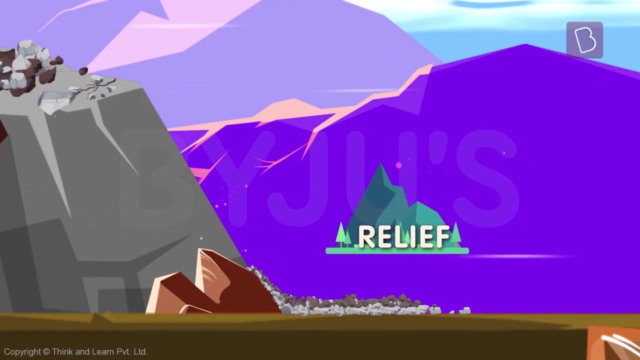 disintegrate into many pieces. This process, called weathering, is the first step in soil formation. The rate of weathering is determined by climatic conditions of a given place. The weathered particles either remain there or are transformed. Depending upon the relief or slope, the amount of weathered particles deposited changes. 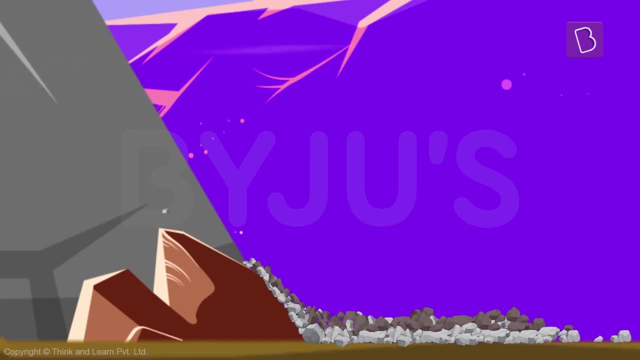 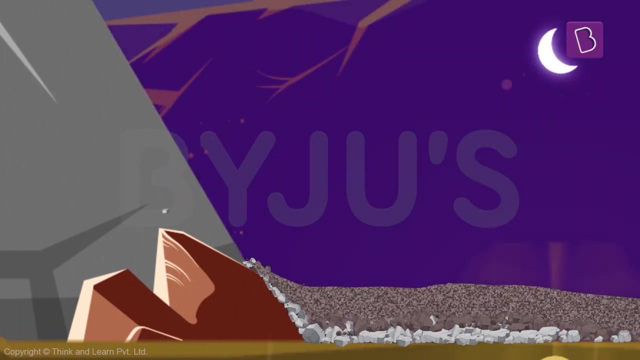 The slopes along a mountain will have thinner deposits as erosion is more on slopes, while foothills or plains will have thicker deposits. Over time, more and more weathered particles accumulate, leading to an increase in the amount of weathered particles deposited along the slope, reducing the size of the exhaust. 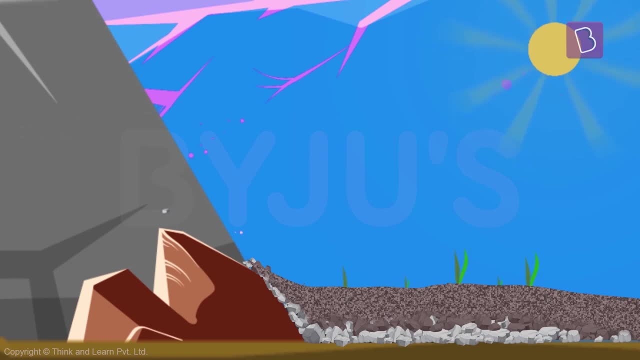 The soil remains as it is for several decades. Although the soil remains for several decades, european soil remains as it is for the next ten decades. The soil is still more fertile than in ancient times. The soil remains as it is for 30 years. 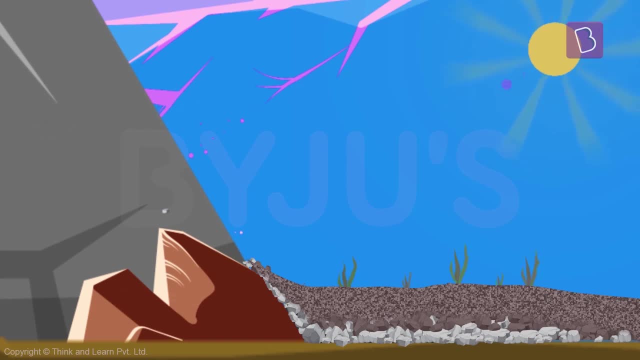 In the last century, more than a century of efforts were made to clean up the soil and clean it up. Plants and small organisms grow, mature, die and become part of this soil, adding to the humus content of the soil. Thus, parent rocks, climate relief or altitude or slope, flora and fauna and time are all 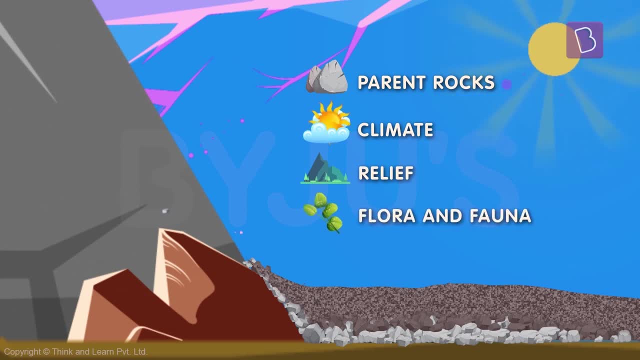 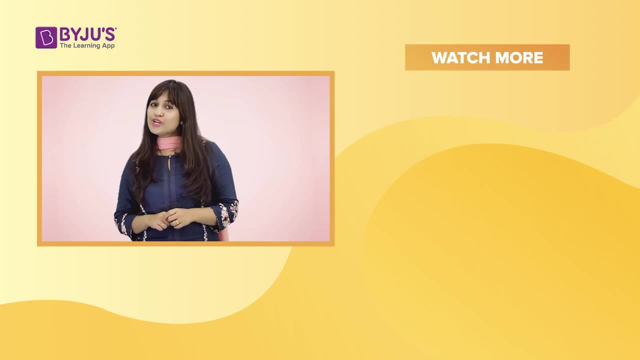 active and present at the bottom of the soil. The soil is a good source of water. The soil is a good source of temperature and moisture. A soil that is gentle to the spot and frequently unclean from underground air is considered one of the and time are major factors in soil formation.